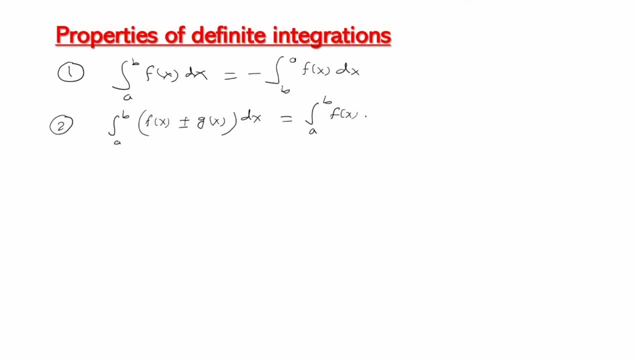 as a to b, f of x, f of x, dx, plus or minus a to b, g of x dx. third property is the additive properties. so sometimes we need to break the integration into two part and this rules is helpful for that. a to b? f of x, dx can be written as a to c, f of c to b, f of x. 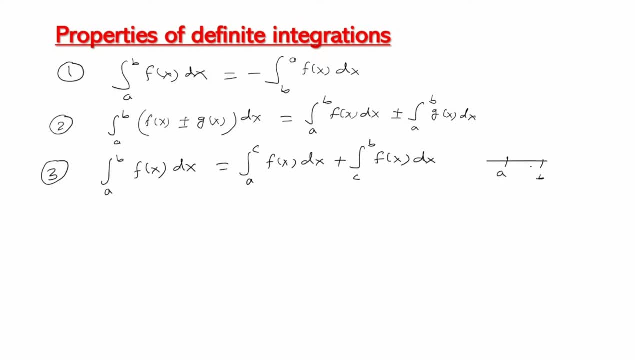 dx, where c is a, any middle point between a and b. the fourth is the constant multiply a, b k of f of x dx. in this case we can take out the k and we'd have a to b f of x dx. and the fifth is a to a f of x dx, which will be zero. 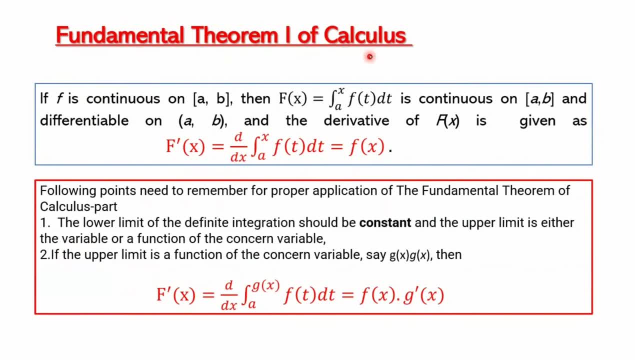 next is the fundamental theorem, part one of calculus. so this theorem state has, if f is continuous on clause interval a, b and a capital f? x is defined as integration a to x, f of t, dt, which is also continuous on a, b and different level on the opposite, interval a, b and the derivative of f x is given as: 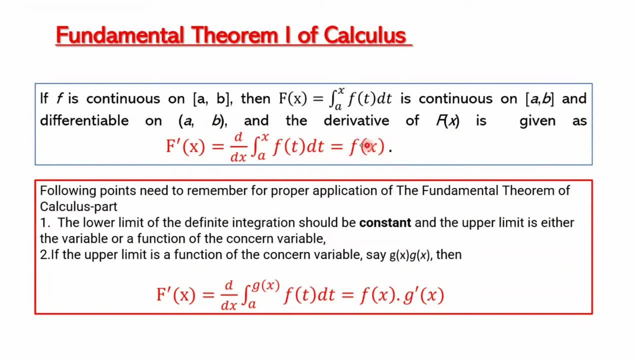 d, dx of a to x, f of t, dt, which is equal f of x. here need to be noticed that the lower limit is a constant number, upper limit is the variable same of these functions. then, derivative of this capital, f, x is same as the integrand the function which we are doing, the integration. 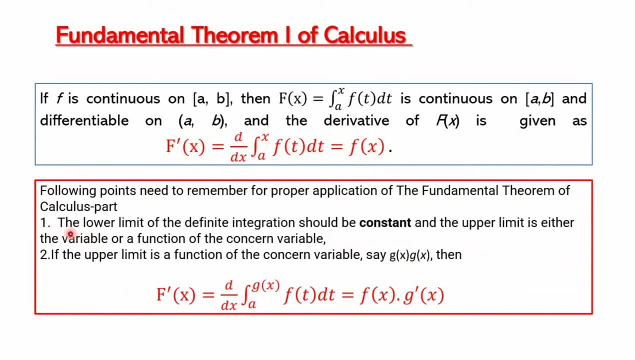 same. so these are the two points. we need to remember it. the lower limit of the definition should be constant. if it is not, means if the upper one is constant, one one is the upper one. that means it is some function of x. now, if this is the variable, we know how to change. 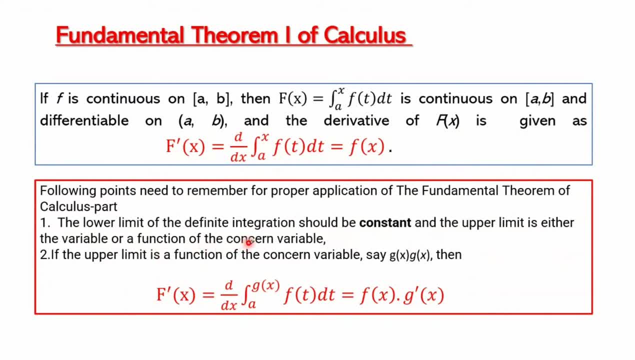 it using the properties of the definite integral. so the upper limit is either the variable or a function of the concern variable. if upper limit is a function means if it is not, x is some function of x. then we have to find. the derivate is like this: f, dash, x is equal d, dx, a to g, x, f of t. 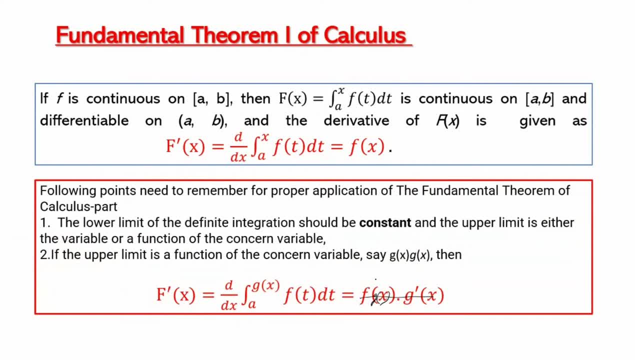 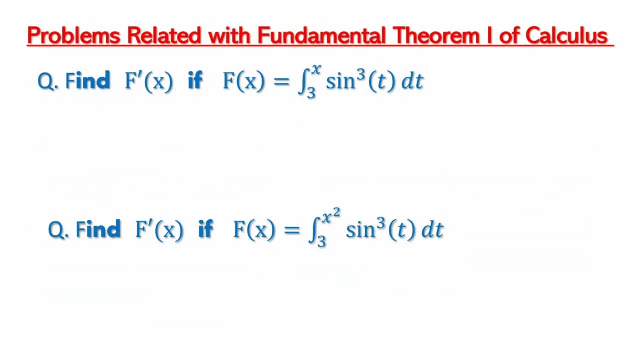 dt. it will be F of G, X and then derivative of G. now we will apply the fundamental theorem, one, and we'll solve this problem. find M does X if FX is equal to 2x sine 3 T DT. so it's simple, by directly. so M does X is equal. that's all now in this. 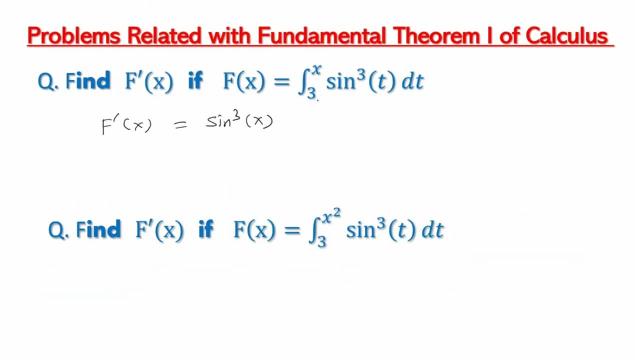 case. here you have, instead of X, it's X square. so look on the difference between this two problem: here it is X, it is X square. that means function of X. so in this case we have to do one step more. M does X. this is equal D. DX of 3 to X square, sine 3 T DT, which is equal sine. 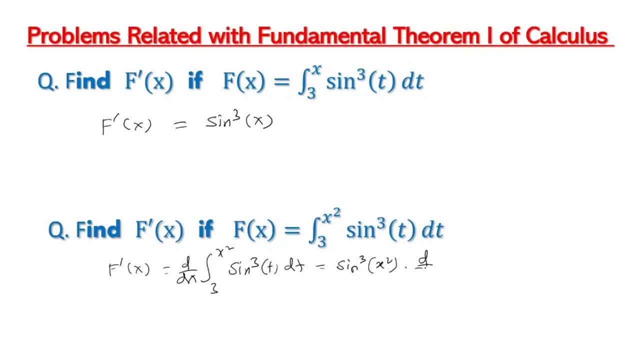 to the power 3 X square and the derivative of X square, so, which is equal to X sine to the power 3 X square. that's all. now we have a another problem where you have the upper limit is constant, lower limit is a function of X. so in this case, before solving the 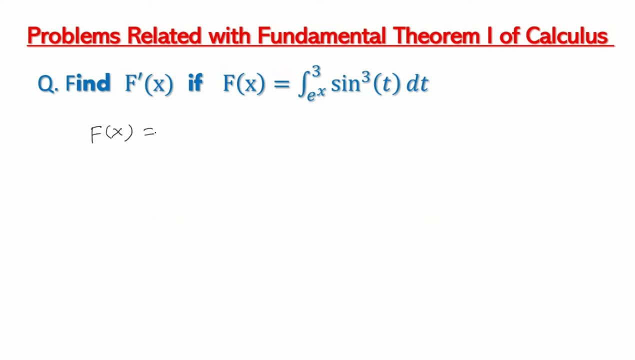 derivative. we need to rewrite it because in our standard form we must have: the lower limit is constant and upper limit is variable, or honden of the variable, so it can be written into combination three. so this is 진 result we have. now we have. we must reduce this to zero, so it will be be equal to three. so now here we need. 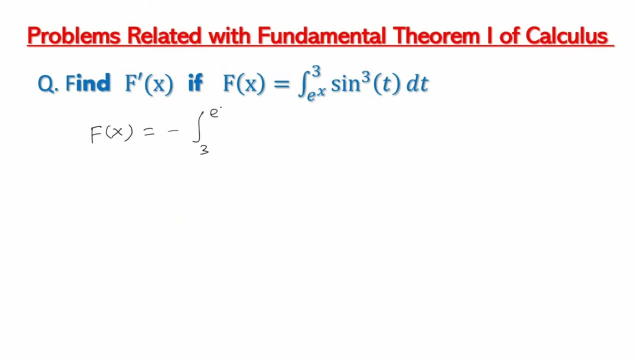 as minus 3 to e to the power x, sin 3t dt. So this implies the fundamental theorem f dash x is equal minus as it is sin power 3 e to the power x and then derivative of e to the power x, which is equal minus e to the power x, sin 3 e to the power x. 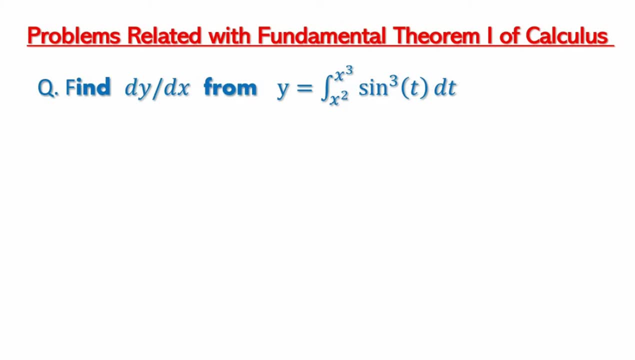 Now, in this problem we have both limit or variable, x square and x to the power 3.. This problem can be solved by two methods. One is we can write this y as say, x square to 0 dt plus 0 to x to the power 3 dt. So 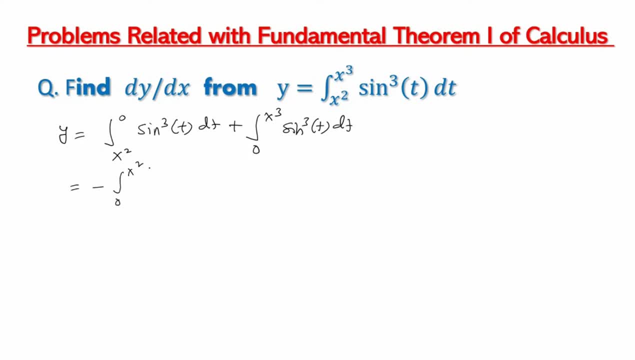 this can be written as: minus 0 to x square 3t dt, plus 0 to x to the power 3.. Now we will apply the fundamental theorem, So dy dx is equal minus sin 3 x square derivative of x square plus. 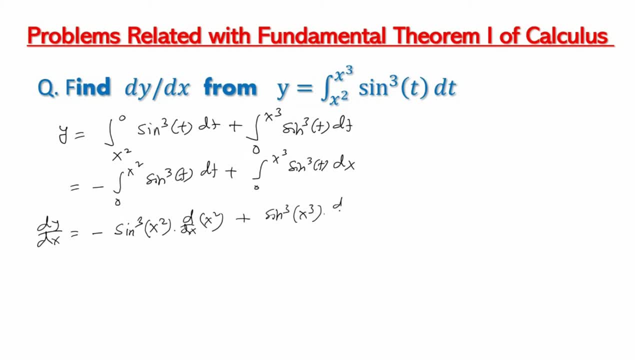 sin 3 x cube plus derivative of x cube, So which is equal minus 2 x. sin 3 x square plus 3 x square, sin 3 x to the power 3.. This method can be summarized as: whenever you have y equal to 1 minus x to the power 3 or x to the power 2, because x square is equal to, 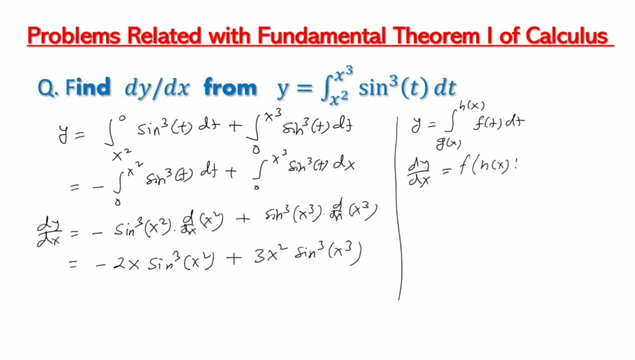 0. So this is like this. Let's see what I've written. Let's say y is equal gx, hx, f of t, dt, then dy, dx. we can have f of hx, h dash x minus, f of gx, g dash, x minus. Значит y is equal to the power 3. 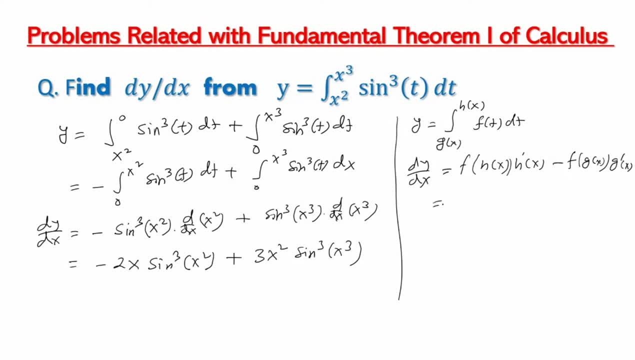 and the value of y we will use, So that will be X. so in this case this is equal sine 3 X to the power 3 derivative of X to the power 3, minus sine power 3 X square, derivative of X square. so this is equal. 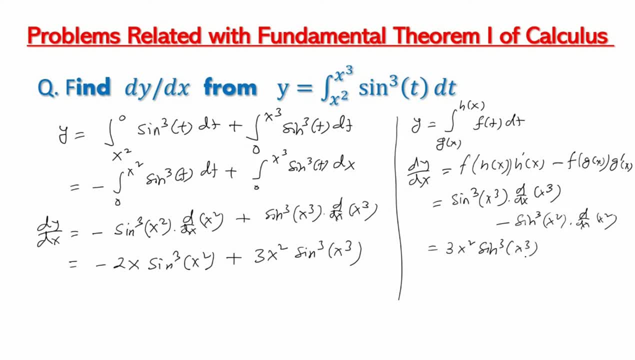 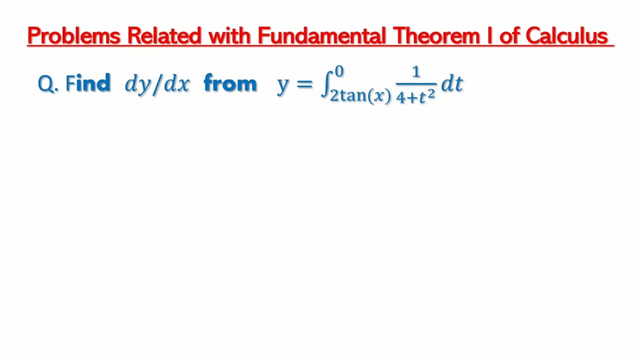 3 X square X to the power, 3 minus 2 X sine 3 X square. so both the way answer are same. the next one is: dy dx from y equals the 2 tan x to 0, 1 over 4 plus t square dt. so again in this case we need to reverse in order of: 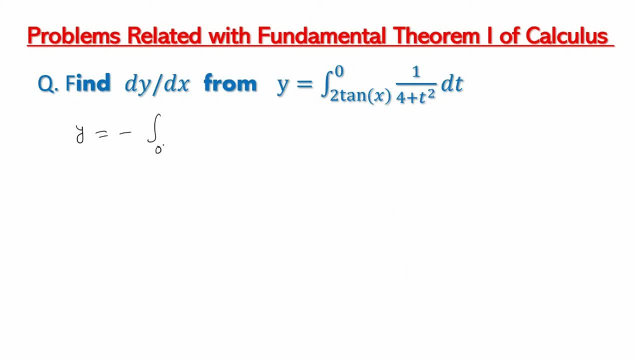 the limit. so y is equal minus 0 to 2 tan x, 1 over 4 plus t square. by fundamental theorem this implies dy dx is equal minus 1 over 4 plus 2 tan x. whole square then tdx of 2 tan x. so this is equal minus 2 second square x. 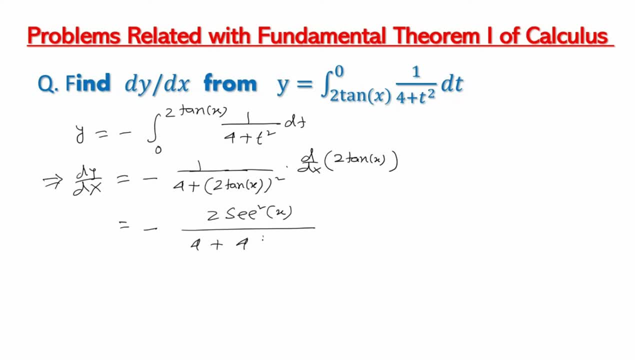 this will be 4 plus 4 tan square x. so this is equal minus 2 over 4. second square x over second square x. here we are using 1 plus tan. square x is equal to second square x, and here we are using derivative of tan. x is equal second square x. this is equal minus half. 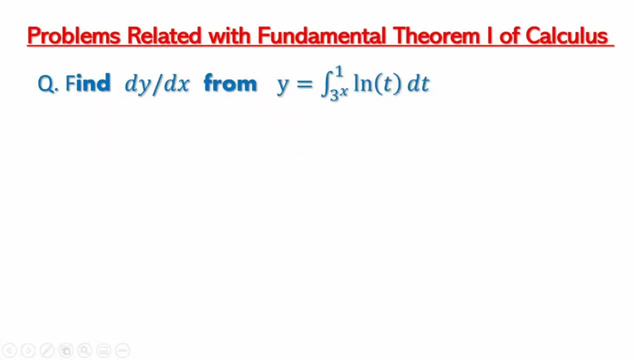 the last problem on this section is: y equal 1. y is equal 3 to the power x 1 lan t. so again you have to write it first. y is equal minus 1, 3 to the power x lan t, dt. so dy, dx. this is: 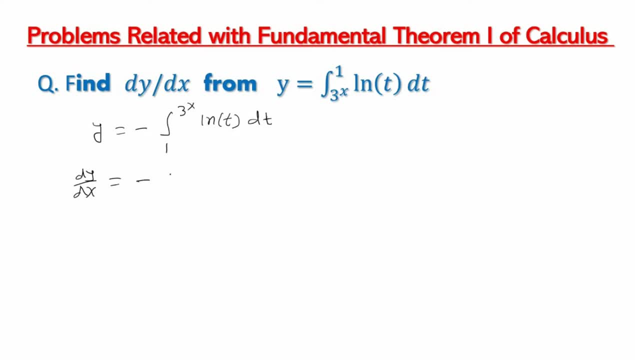 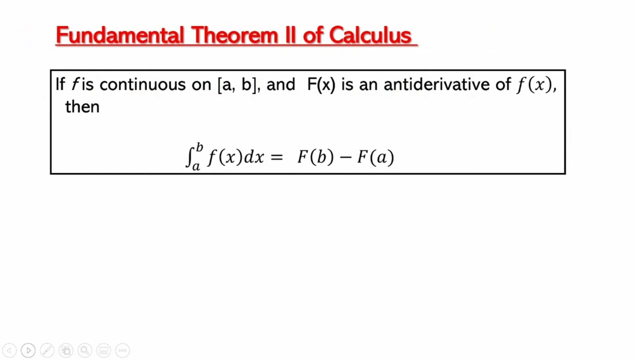 equal minus lan of 3 to the power x, derivative of 3 to the power x tan x. so this is equal minus x and derivative of 3 to the power x is 3 to the power x lan 3. next we have fundamental theorem 2 of calculus. so in this case we have: 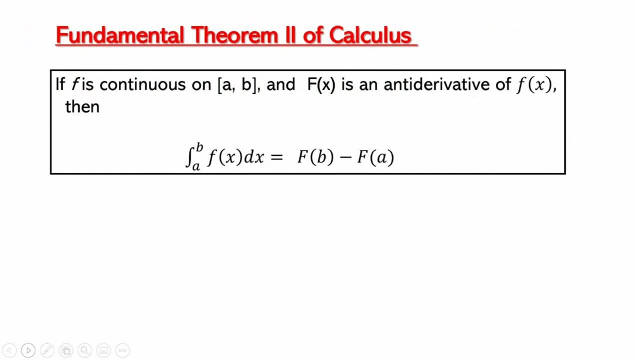 exactly the idea that how we will do the definite integration. so you see that if f is continuous and fx is an antiderivative, so for this, to apply this theorem, we must know the anti-derivative of the given function. then we'll have a to b, f XD, x is equal. f of B minus F of a will do more example. 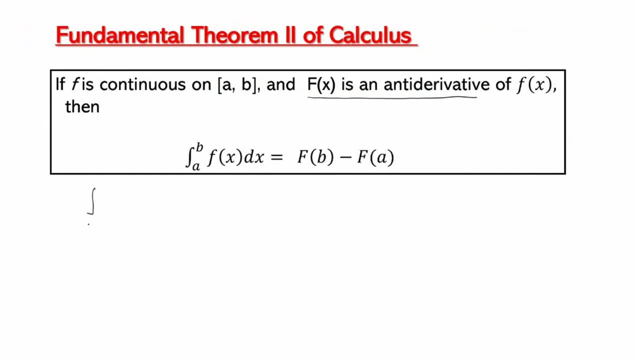 but let's add the sample example. suppose one to two X DX equals two d x. we see that this fx is ROBERTAM, The anti-derivative of condemnable function of the specimen. he align its development future. we'll not calculate it for 후 monstersaphon. 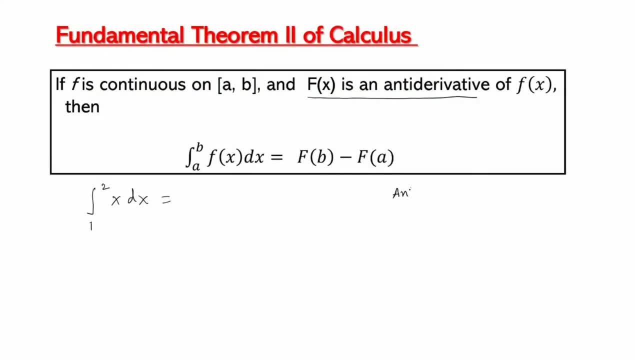 so we know that the antiderivative of x to the power m is x to the power m plus 1 over m plus 1. m is not equal minus 1, so in this case m is equal 1, so we will have the antiderivative is: 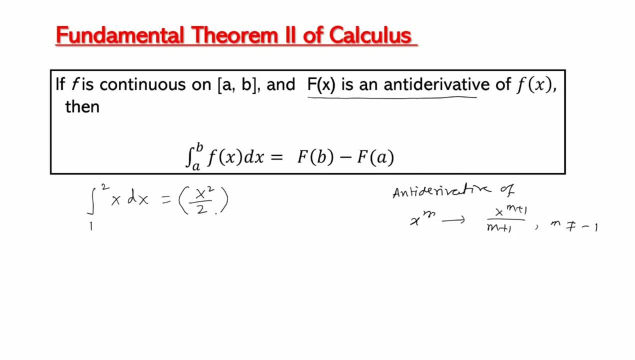 x square over 2 and the limit is 1 to 2. so this is equal upper limit. so 2 square over 2. so this is f of b minus f of a. so this is 1 over 2. so this is equal 2 minus r. so this is. 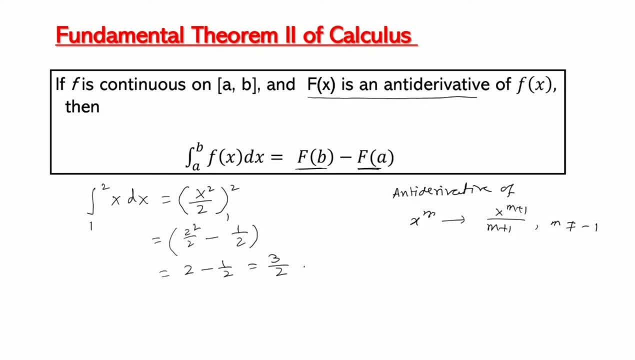 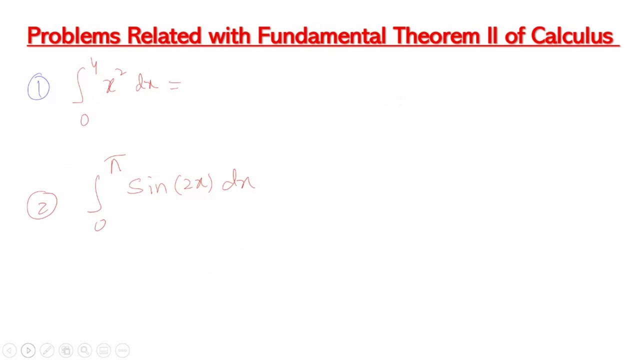 3 over 2. so therefore, the indication to, therefore, to use the fundamental theorem, part 2, you should know the antiderivative of the answer. so now we will consider different problems and for this part, at this, at this moment, you should know the antiderivative of each of the functions. then you 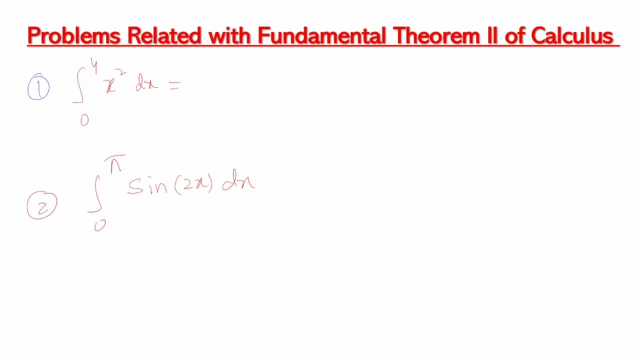 can solve it. so first problem is we have x square dx, so in this case the antiderivative is x to the power 3 over 3 and limit is 0 to 4. so upper limit 4 to the power 3 over 3 minus 0, that means 64. 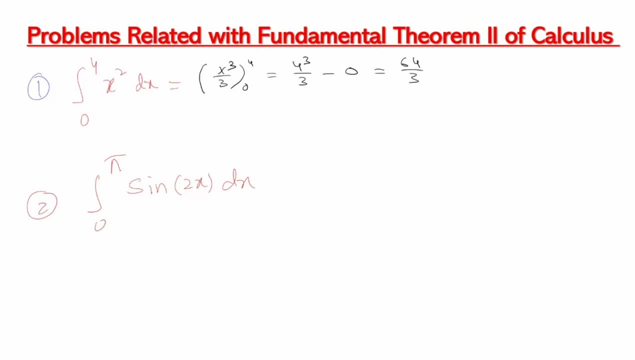 over 3. this is the answer. so for the definite integral there will be no constant c and the answer will be always numerical number, now antiderivative of sine 2x. so we know that d dx of cosine 2x over 2 minus is equal sine 2x. so therefore the integration is: 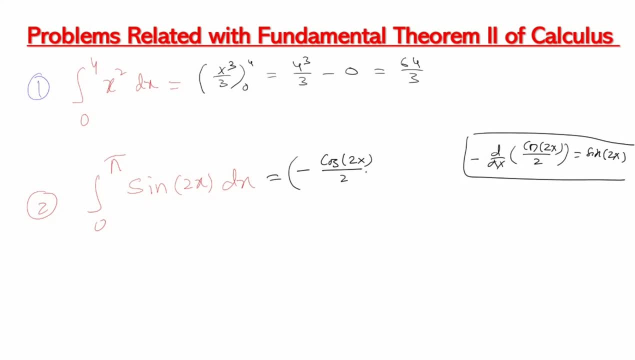 minus cosine 2x over 2 limit is 0 to pi, so this is equal. take out the minus half first and then 0 to 2x 0 to pi, so this is minus half cosine 2x over 4. so in the first two cases you want to have a constant of c one, two materials, so 1 plus theta, square one plus zero here. 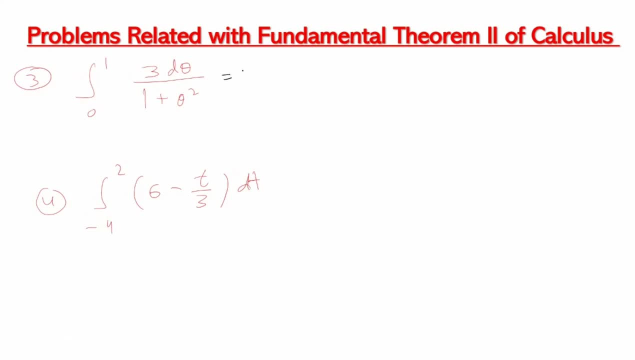 every set of ungefheavy elements in first is equal to 0, and in second case you will have a constant of 1 along with zero. two can take out and then you have 0 to 1 d theta over 1 plus theta square. we know that d d theta of. 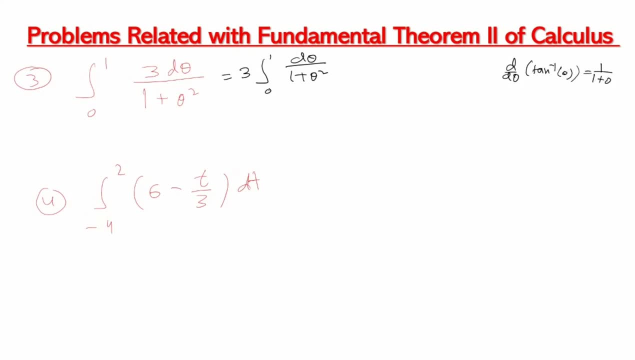 tan inverse theta is equal 1 over 1 plus theta square, so this is equal 3 tan inverse theta. limit is 0 to 1, so therefore this 3 tan inverse of 1 minus tan inverse 0, so this is 3 pi over 4 minus 0, so the answer is 3 pi over 4. 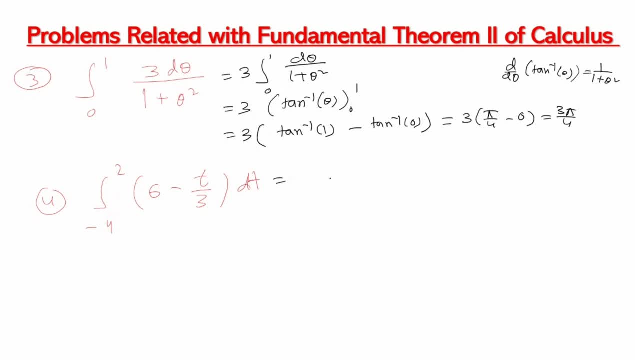 so this problem, you can do either separate them as a two function or two indication, or you can do it together. i will prefer to do it together. so the first one is 6 and dt, so it will be 6 t minus t. the antiderivative will be t square over 2, so it will be 1 over 6. 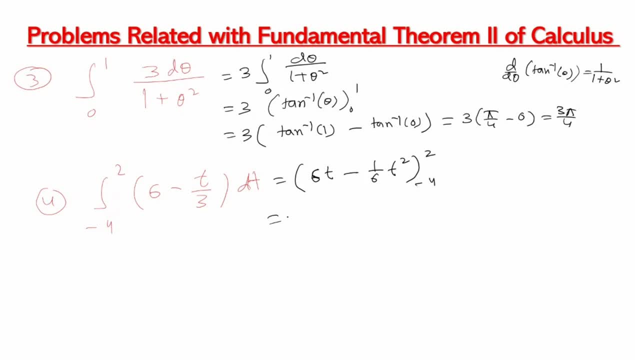 t square limit is minus 4 to 2, so i will put the 2 first, so it will be 12 minus 4 over 6, then minus minus 24, and then minus 16, so 12 plus 24, so 36 and minus 4 over 6, plus 16 over 6, so which will be? 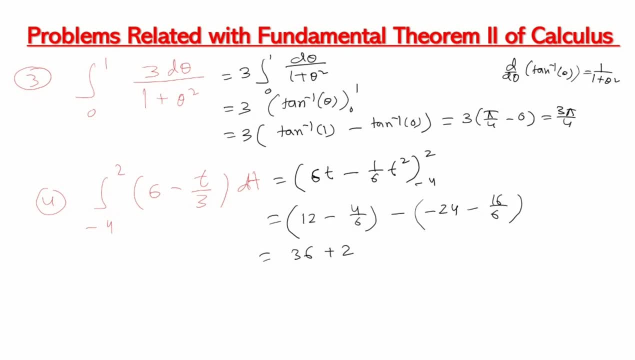 plus 12 over 6, so that means 2. so this answer is 38. here again, you can do separately or you can do togetherly, so i'll prefer to do together. so 3 x squared, so it will be 3 x to the power, three over three minus two. 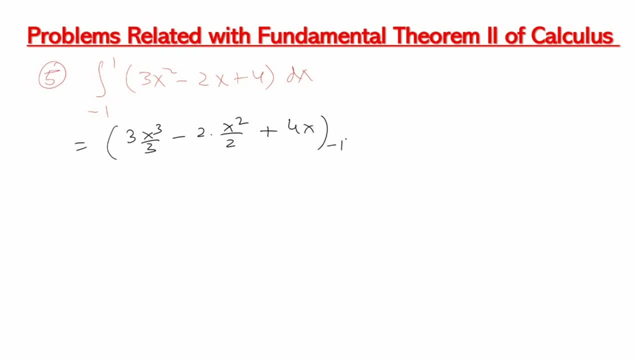 x square over two plus four. x. limit is minus one to one. so this is x to the power three, 3 x squared加 445. 3 x square over 3 plus 4 x. we're going to divide by 2, so it will be 6, and terms equal to 2, and that will be –4 to 1. so 3 x to the power 3 –x square over 2 plus 4x. limit is minus one to 1. so this is x to the power. 3 minus x squared plus 4 x limit is minus 1 to 1. so this is x to the power 3 –x square plus 4x. Tim Shiona to. 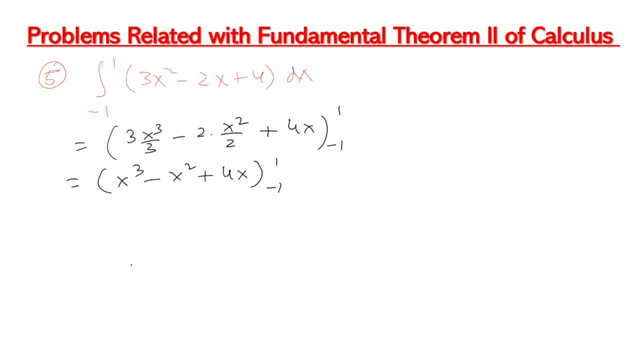 minus x square plus 4x minus 1 to 1, so this is 1 minus 1 plus 4, minus minus 1. minus 1 minus 4, so this is equal 4. this is minus plus 6, so this is equal 10. 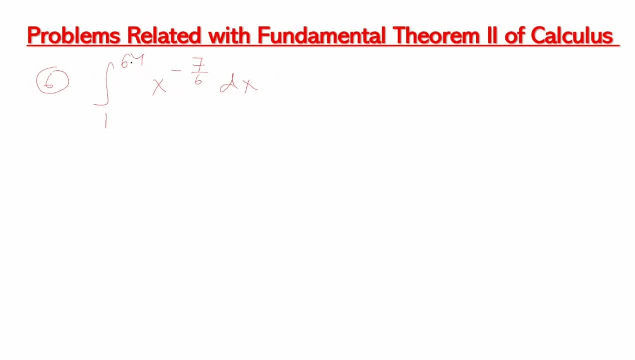 plus it is 1 to the 1 to 64, x to the power minus 7 over 6. so again, so it will be x to the power minus 1 over 6, 6 to the power minus 1 over 6, minus 1 over 6, 1 to 64. so this is: 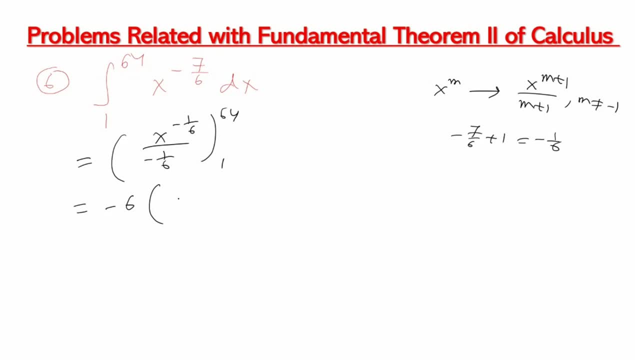 equal minus 6, 64 to the power minus 1 over 6 minus 1. so this is equal minus 6, 64 to the power minus 1 over 6. so 60 to 4 is equal 2 to the power, 6, 64 to the. 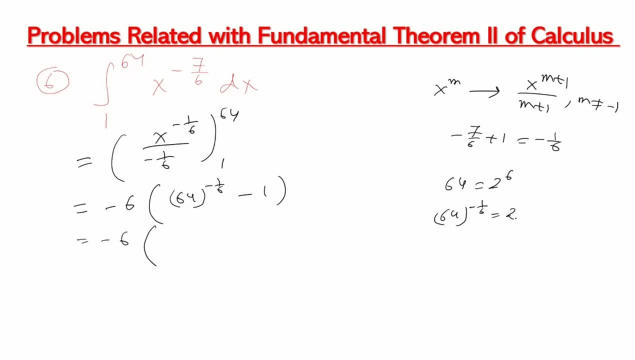 power minus 1 over 6 is 2 to the power minus 1. this is equal half minus 1, so which is equal 3. next problem is 0 to 2 pi 1 plus cosine x over 2 dx. so here we can do it like: 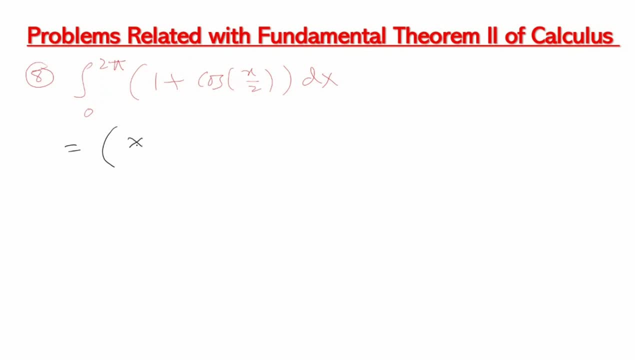 this and the derivative of dx is equal x plus sine x over 2 over half, 0 to 2 pi. so this is equal x plus 2 sine x over 2, 0 to 2 pi. so we'll first put the limit: 2 pi, so 2 pi. 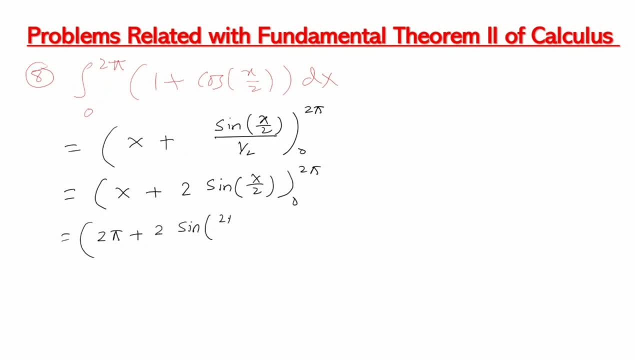 plus 2 sine 2 pi over 2 minus 0 plus 2 sine 0, so it will be 0, so this is 2 pi 2 sine 2 pi over 2 minus 0 plus 2 sine 0, so it will be 0, so this is 2 pi. 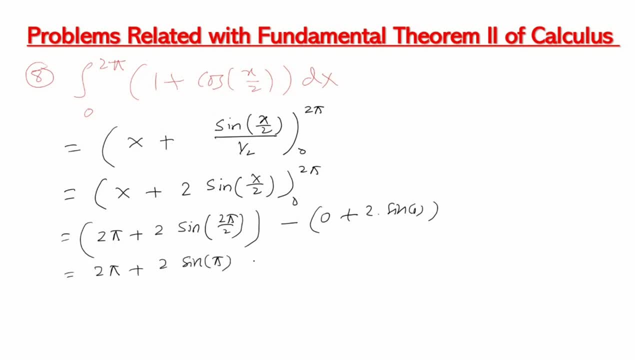 plus 2 sine pi, so this is equal to pi. so to solve this problem, let's recall: d: d theta of second theta is equal second theta 10th. so therefore, for this function, the anti derivative is second to you. our second to you over to the limit is 0 to pi over 6, this is equal half second.